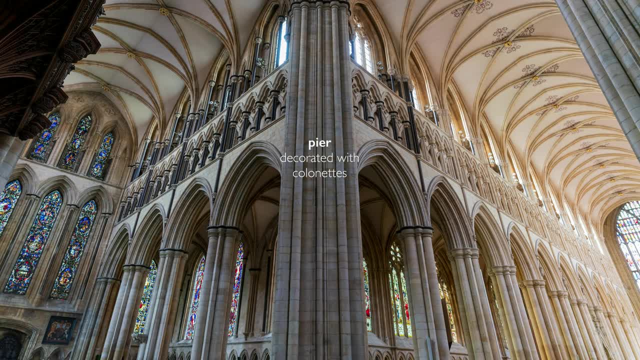 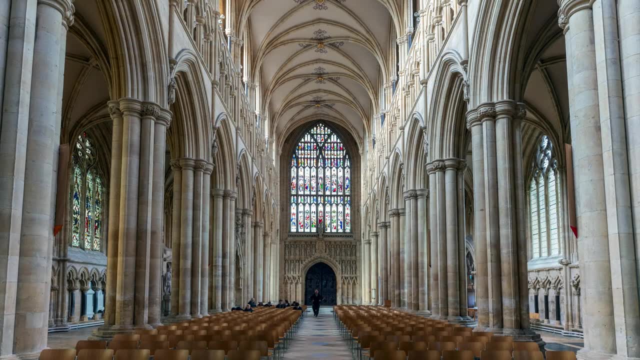 But this was a massive object that helps to support the stone vaulting above. But there's another structural system that's at work. Even with the pointed arch, the vaulting of these churches still created lateral thrust that pushed outward, And so the building had to be contained. 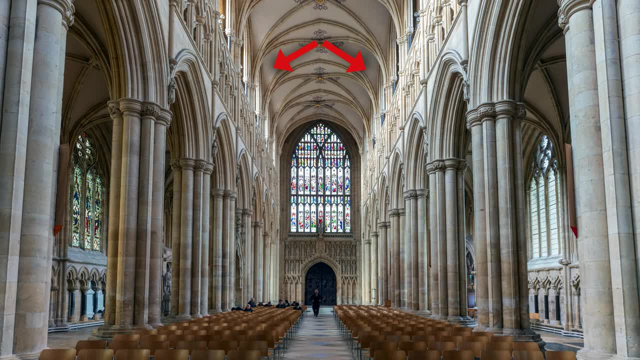 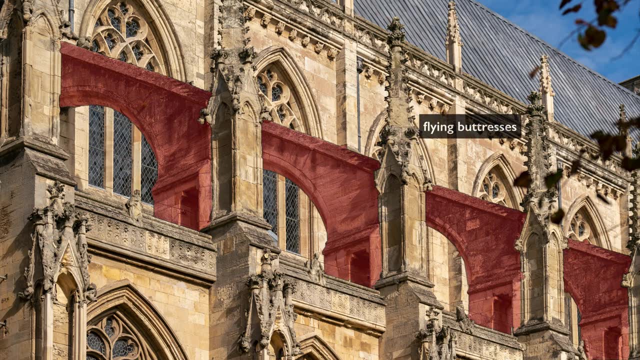 It had to be supported from the outside. It had to be buttressed, And that's where we see one of the great features of Gothic architecture: the flying buttress, essentially a bracing in between the windows on the outside of the church. 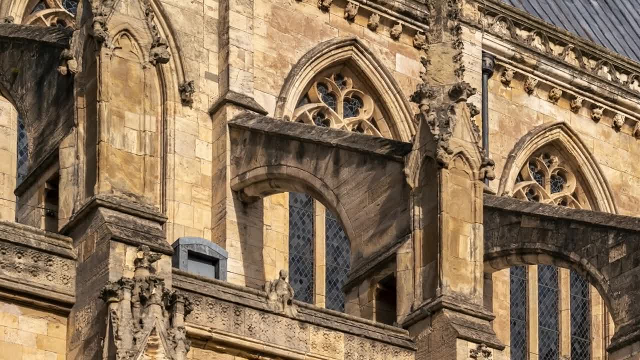 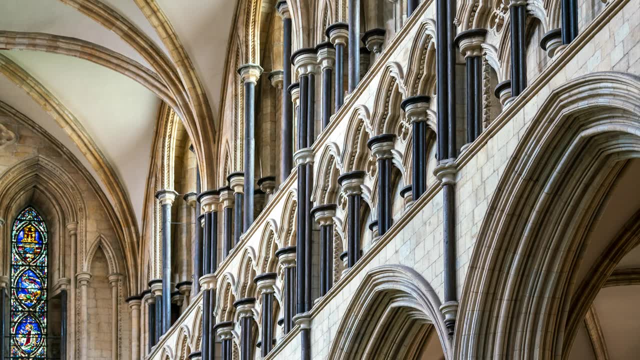 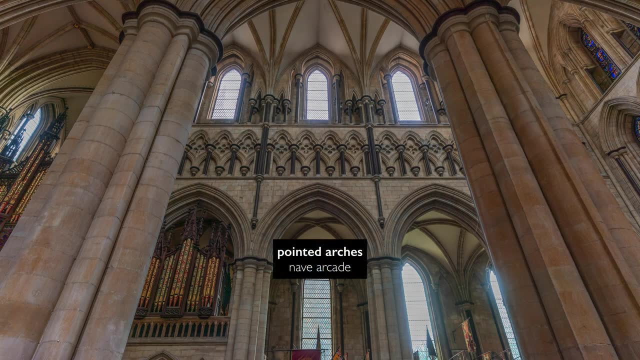 And because they are relatively delicate and pierced, they allow light to get to the windows, to flood the interior with brightness. When we look up along the wall of a typical Gothic church we usually see three parts. We see the pointed arches that form the nave arcade. 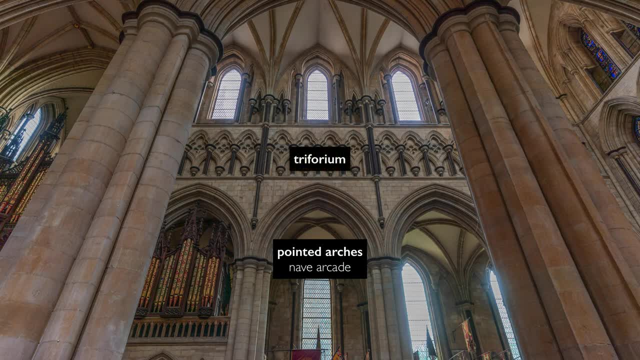 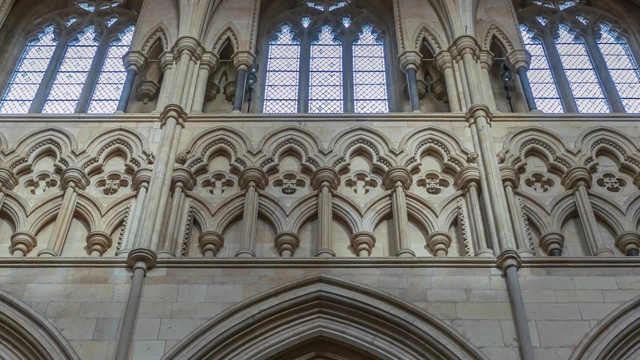 We see above that the triforium And then above that the clerestory, the level with windows. When we look at the triforium, even there we see the wall is pierced. Here in Beverly Minster we see trefoil-shaped arches. 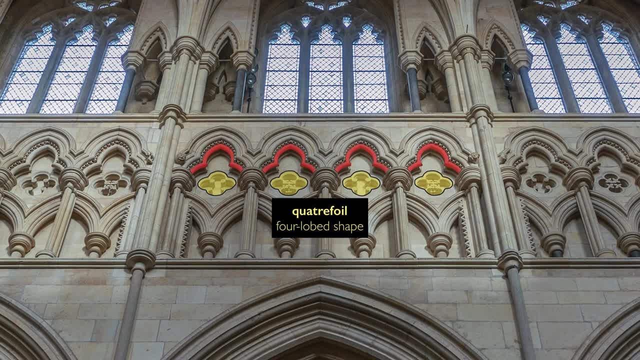 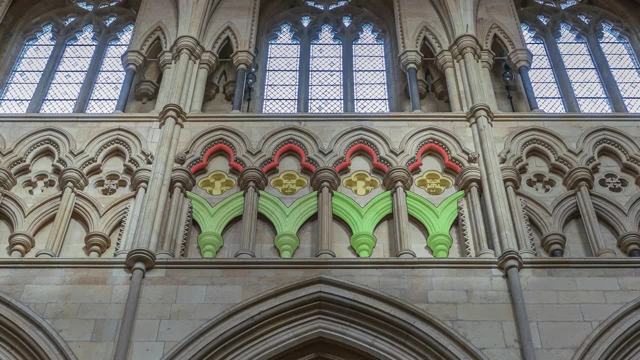 And within that trefoiled arch we see a quatrefoil, And then, below that, yet another level of opening of these short pointed arches that are separated by columns. So this layering that allows the wall to have a sense of depth. 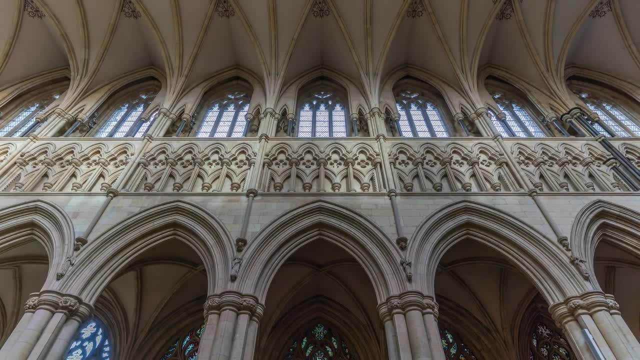 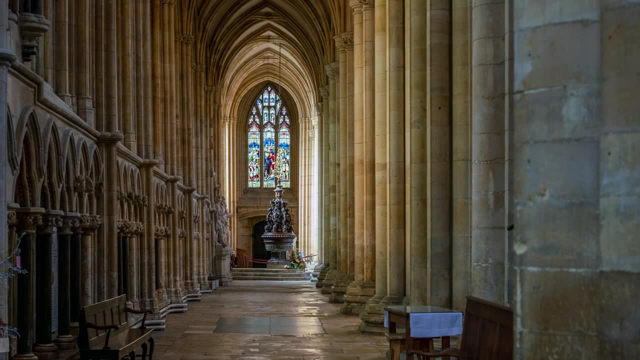 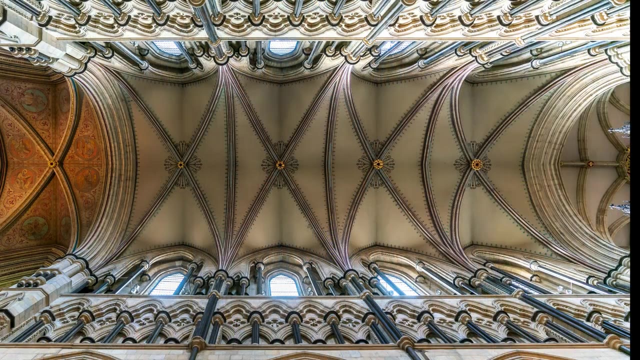 All of this brings our eye upward. It emphasizes the heavenly. The intent of the Gothic church is to create a sense of the heavenly on earth. If you imagine a typical person's home in the 13th century, we imagine something rather dark and without a lot of windows. 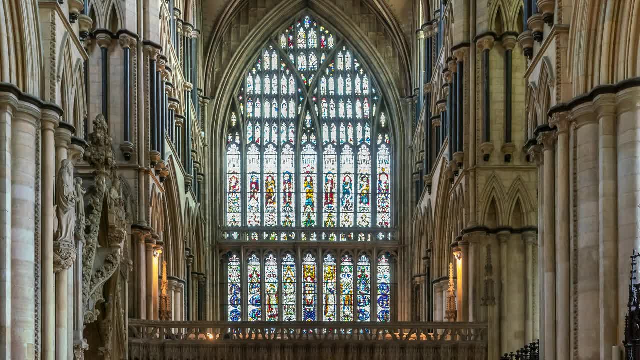 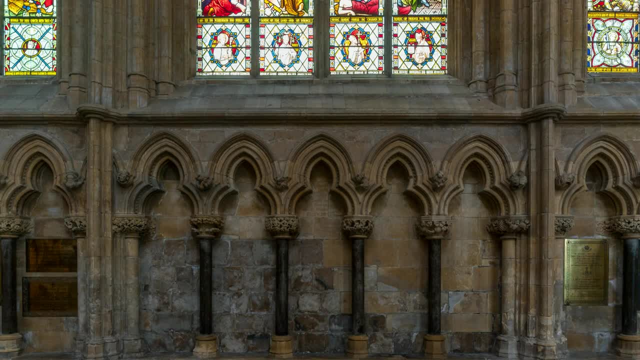 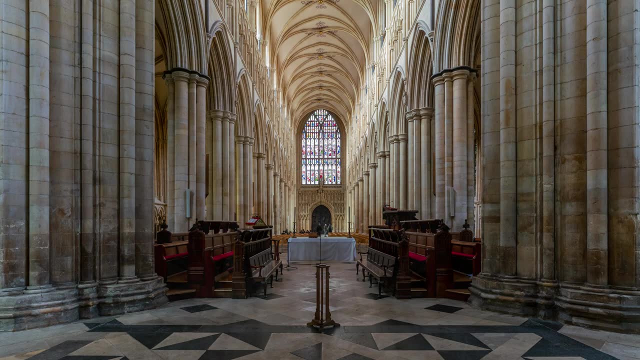 And so coming into a space like this must have seemed truly miraculous. It's even difficult, I think, for us in the 21st century to imagine the workmanship, the decades of labor and the enormous costs that went into these buildings and these places of worship. of places of connection to the divine.